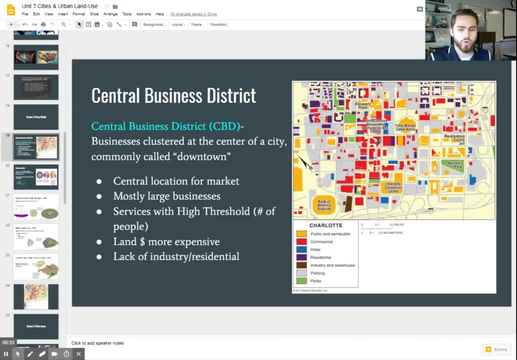 tall buildings in this general location, And it's not a whole lot of residential dwellings. Now there may be some interspersed between different types of businesses, but most of it are large scale businesses that build vertically right. There's not a lot of space here, And so in order to maximize that central location, they have to build upwards, And that's why you start seeing skyscrapers in the center of cities, And so this is a central location. 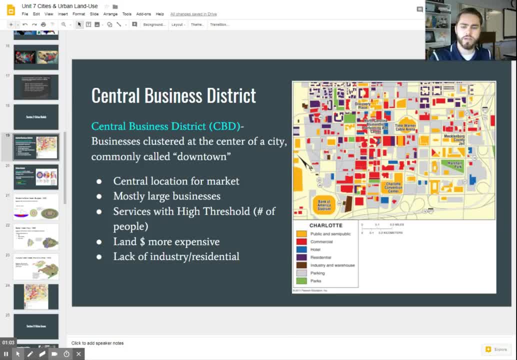 The central business district or downtown area for a particular market. So remember, we're talking like in central place theory. there's a central market where people will travel to, And that's the same for large businesses. You know, you take a look downtown Charlotte, you have the Bank of America building downtown And you see that you know people will travel from all around Charlotte to get to that particular area for work. And so there's a 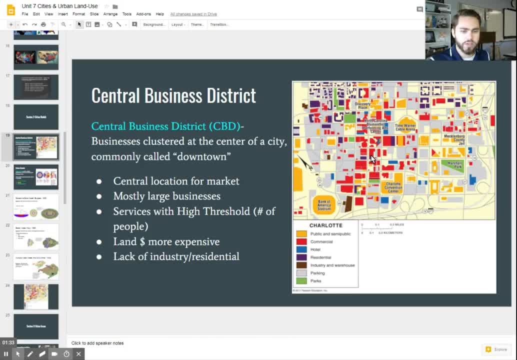 large number of people to draw from if you put it in that central location. So no matter where you put it, you know you have equal distance. whether you're on the north side, the east side, the west side, you can draw from all the people in that general range. All right. And so we also see stores and businesses with a high threshold that we talked about in central place theory, So ones that require a large number of people to sustain it. All right, because that central location has the most people. 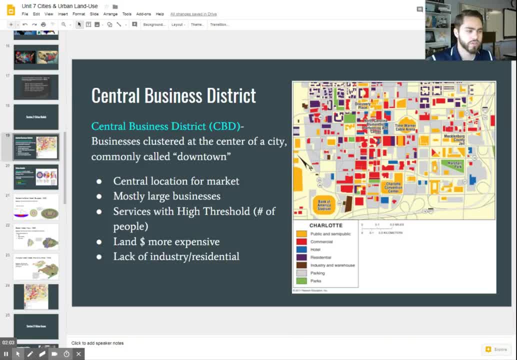 surrounding that particular business. We also know that land is going to be more expensive at that central area. So that's why- another reason why businesses start building vertically in that central business district. There's not a whole lot of land to go around and the less of something makes it more valuable. And so they start building higher and higher buildings on that particular lane. And we start noticing that you know, other types of places cannot afford it. The average person can't build a home in a downtown area. So we also know that land is going to be more expensive at that central area. So that's why- another reason why businesses start building vertically in that central business district: There's not a whole lot of land to go around and the less of something makes it more valuable. And so they start building higher and higher buildings on that particular lane. And we start noticing that you know other types of places cannot afford it. The average person can't build a home in a downtown area. So we also know that land is going to be more expensive at that central area. So that 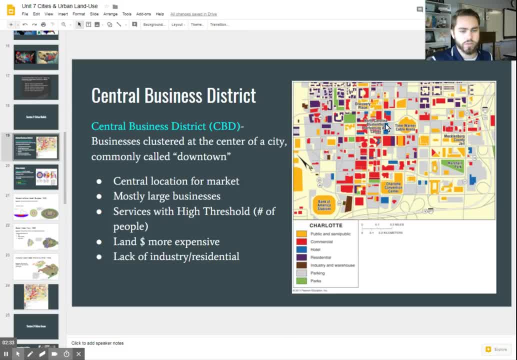 ground to business district, you know, because the lans too expensive, So they'll start moving out. Words start out to that outer ring of residential areas, or maybe even to the suburbs where the lane Is even less expensive. in the same thing for large scale factories. Do factories need to be large in order to produce? 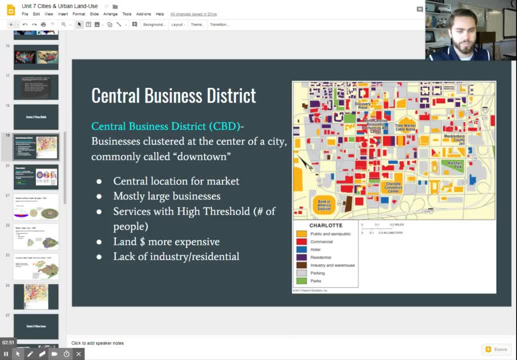 large amounts of materials to have these large machines and so that requires a lot of land and land is expensive in that central business district so they get pushed out to the outer rings as well. so we don't usually see factories and people's residences or homes in that central. 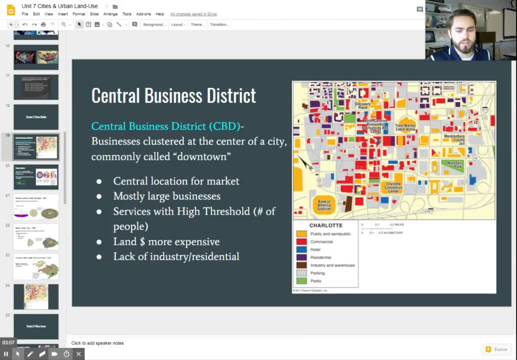 business district. it's mostly large. you know high, high-end businesses or retailers with a very high threshold. so you can see that here in this example of Charlotte as well, that central business district here in the red, not a whole lot of residential downtown, there's a few interspersed, but most of 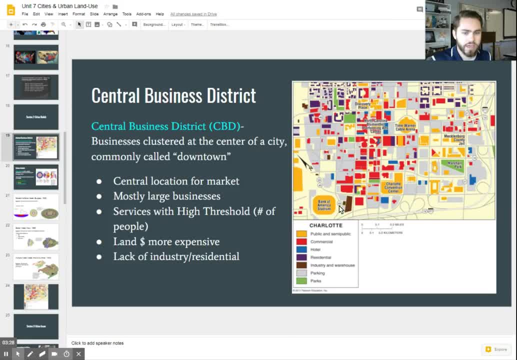 them are around the outside edge. it's the same thing with industry: gets pushed out to the outer edges, where there's more space. so this helps us to understand a lot of different ways in which downtowns are set up. so let's take a look at some of these models that help us to understand the 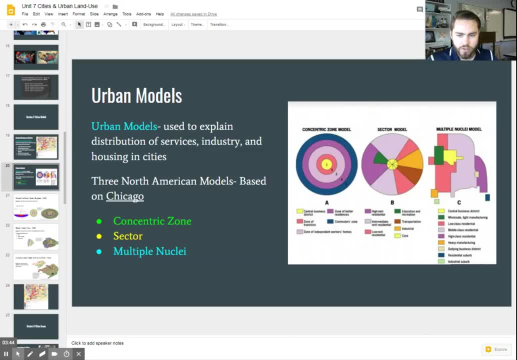 rest of a city. so these urban models were based in North America and particularly based on people's observations of one city in particular, and that is Chicago. these are models used to explain how, in North America, cities are set up. these do not necessarily apply to other parts of the world, and we'll talk 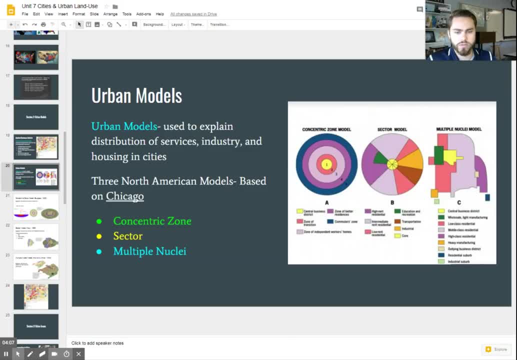 more about that later. but in particularly North America, so you know, especially the United States and Canada, we see that these models apply and the three models help us to understand why we have a central business district and where services, industry, housing, roads and transportation all set up. so let's. 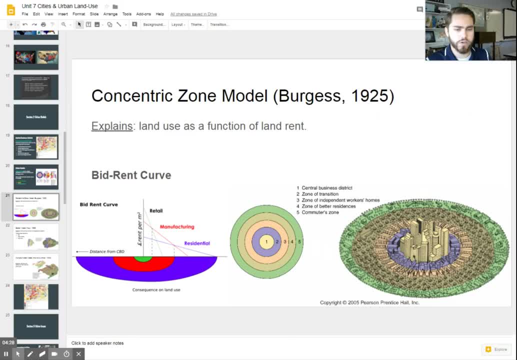 start with the first one that was created by a guy named Burgess in 1925 and that's the concentric zone model. and this is a helpful model that uses the central business district as that center point. we know it typically is located in that central area of a downtown city and what Burgess tend to notice is that 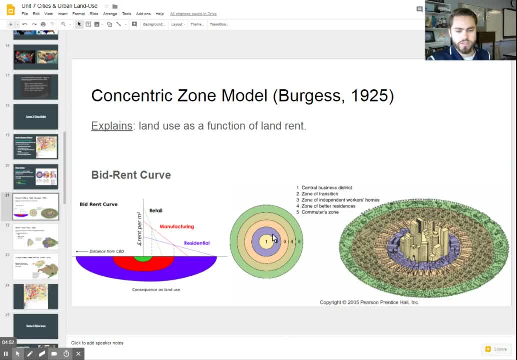 there were rings around that central business district where things congregated, such as in zone two. you have the transition now from businesses to more residential or more factories. so there's, you know, land is a little less expensive, that center area, so they start congregating more houses and businesses. 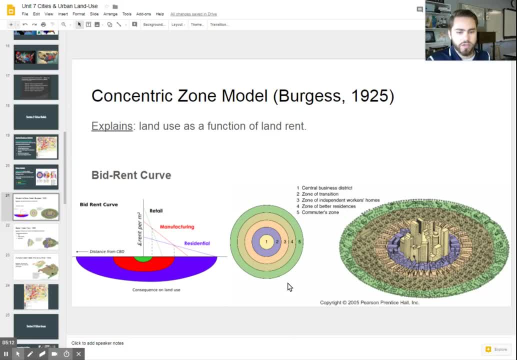 in that outer ring and it's even less expensive out here and we start seeing, you know, more and more houses. but what we tend to notice is that, based on this model is. it explains why that central business district is so expensive. that center point is going to be the land. 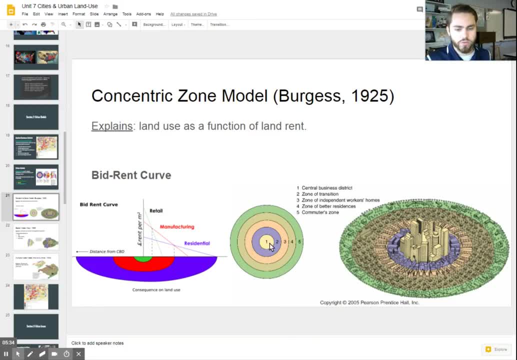 where it's the smallest circle, right. so the smallest circle is right here, in the middle, and so that land there's not a whole lot of it if there's less of something. that makes it more valuable, and so that means that the price of the land in this first zone or that central 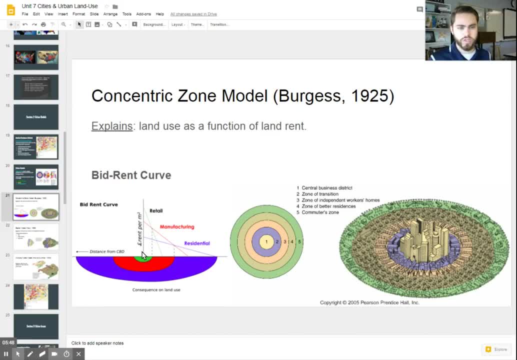 business district is going to be the highest, and you can see that here in this model it's called the bid-rent curve, but basically all you need to know about it is that you know that central part is going to be the most expensive land, and so that's why you start seeing skyscrapers and tall buildings in that. 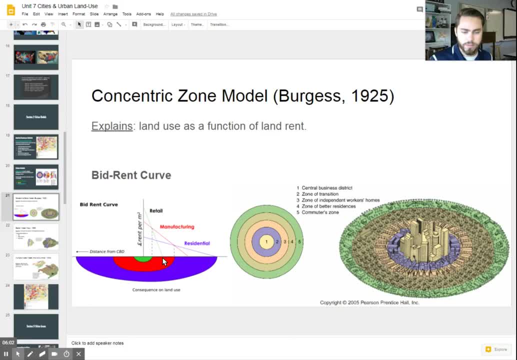 central area and then, as you move away from that center point, land becomes less and less expensive so you can put a factory in there that's a little bit bigger, or some houses or some things of that nature, and eventually you'll see a. you start seeing more and more houses pop up where land is less expensive. 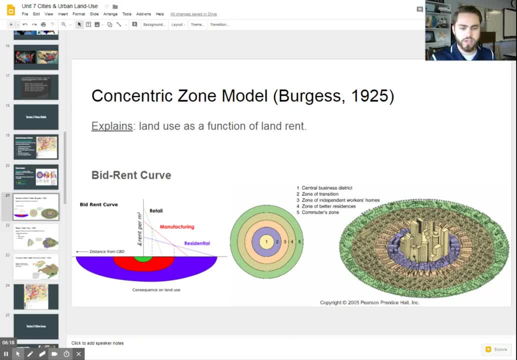 because it's, if you're thinking about it, instead of a business trying to buy land where they have a lot more money, it's just one single person or family trying to, you know, buy a particular house, and so you have to go where the land is cheaper. so we start seeing these rings of residences that surround that central. 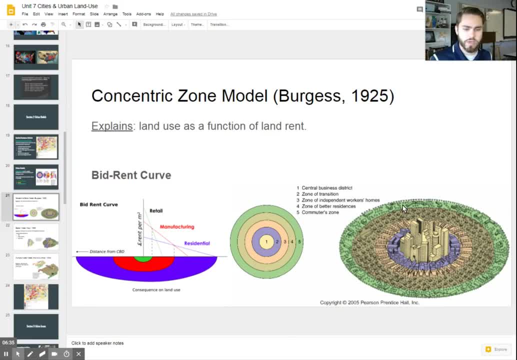 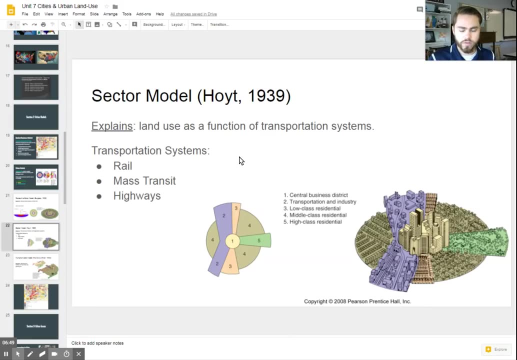 business district and factories, and then the residents surround it, and we can see that here in this bid-rent curve explained by the concentric zone model or Burgess model. all right, and again, this is based off of what he saw in Chicago. all right, the next model is also again based on. 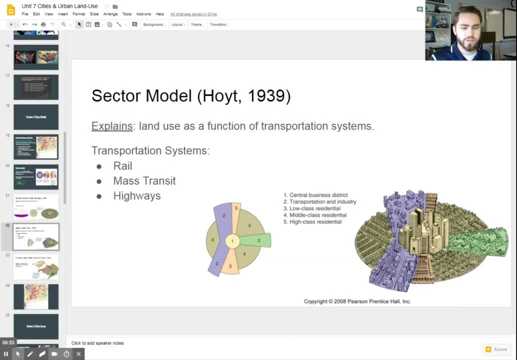 Chicago, but it takes a slightly different aspect or approach to it. you still have that central business district in the sector model, but he Hoyt that is noticed that there were more patterns connected to transportation than there were just simple rings, and this is true especially when roads became more. 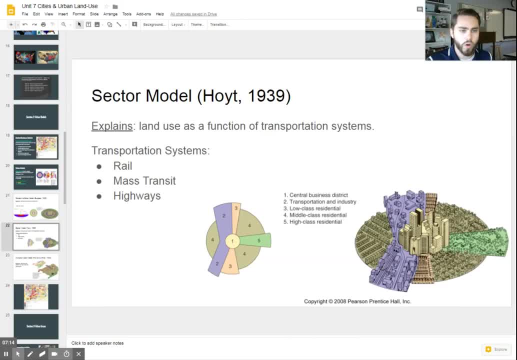 developed and more people had cars and things of that nature rather than walking to work in that central business district, and so they he started to notice that people and businesses congregate around major roads and infrastructure and transportation areas rather than just concentric rings, and so what he noticed is that these are actually little slices cut. 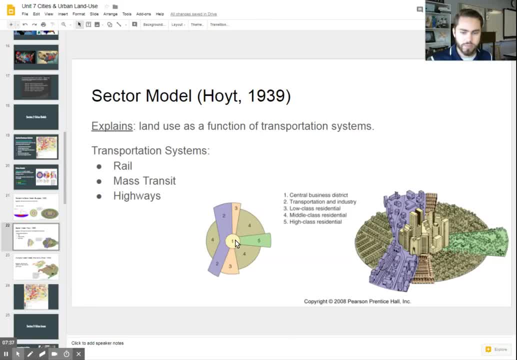 out of the city from that central business district. so notice, you still have a little central business district here in the middle, all right, but now it's shaped more like a like a pie right, or a pizza, where it's got slices of areas that are congregated around. 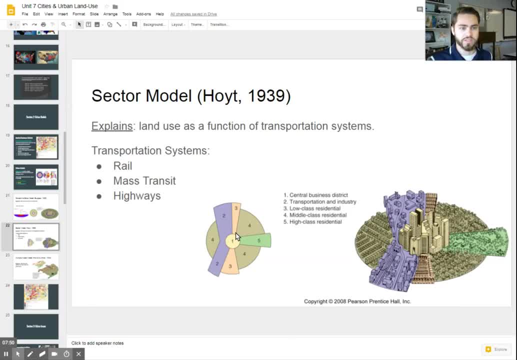 these major roads right? Remember, all roads typically lead to the central business district or there around, And he noticed that you know residences and other industries and things of that nature would center around major roads, because you need people to be able to get around. 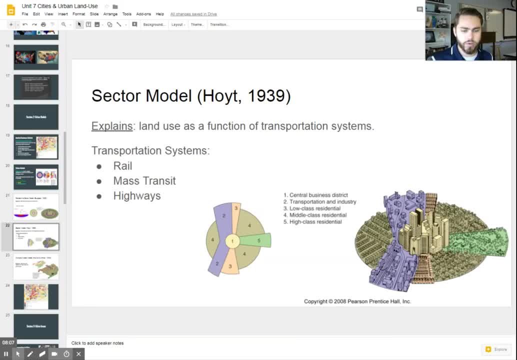 and to. if you're a factory, you need people to be able to bring in resources to your factory, And so you're going to congregate around roads instead, And that's why we also see that there aren't usually major roads that go through areas of residential areas. You have small roads and 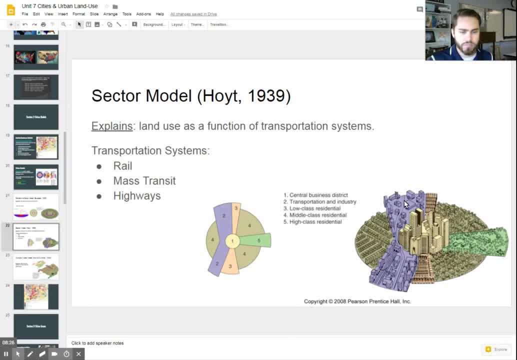 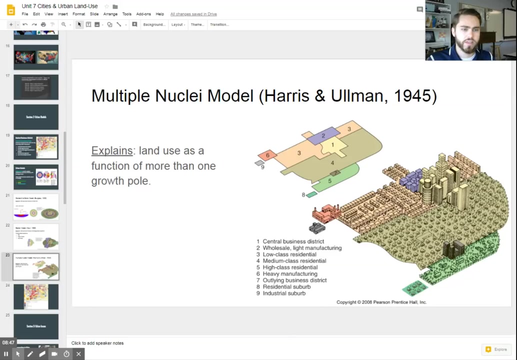 residential areas that you see around here that lead to this major thoroughfare where businesses and factories can congregate to get their supplies in. And Hoyt's model better explains the use of transportation than the Burr. And then, finally, we have the multiple nuclei model. Remember we said that the nucleus of a city 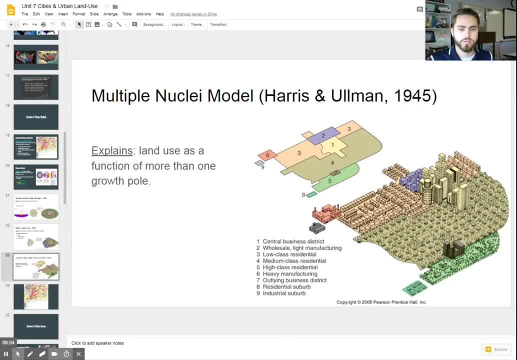 is going to be that central business district. Well, the multiple nuclei model, as you might imagine, is not just one central point but multiple central points And basically what it takes into account is that you know, many businesses have no need at all for the central 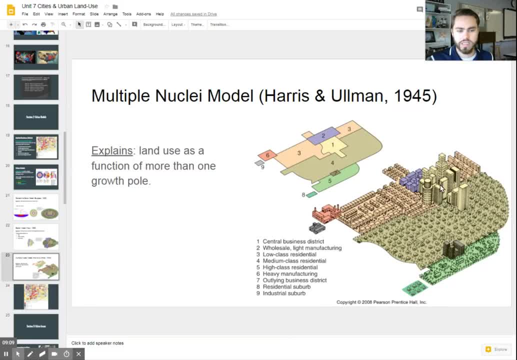 business district right. They're small businesses, they're factories, they don't congregate in that area, So they have their own centers right, And so they have the central business district here. but you have more- you know- industry over here, right In this land. 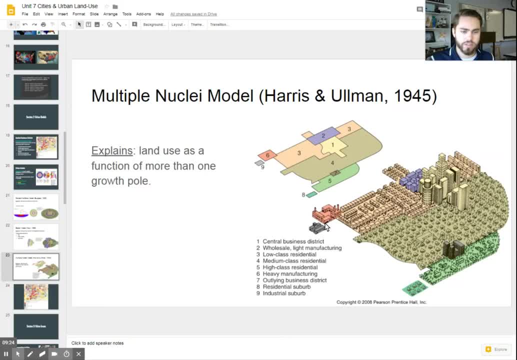 where it's cheaper, And they have their nucleus of industry nucleus over here, And then you have a, you know, light manufacturing or other industrial business over here, And then residences have their own central area where they congregate around over here, And so there's these multiple nuclei. 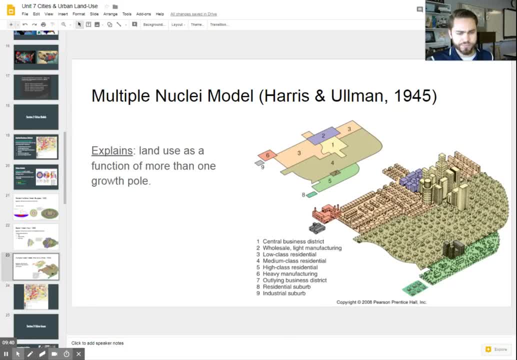 where land is, is grown around, So people congregate around these multiple nuclei rather than just that central business district. So it less emphasizes that central business district and more emphasizes all the different areas where people congregate, So whether it be factories or residential areas, 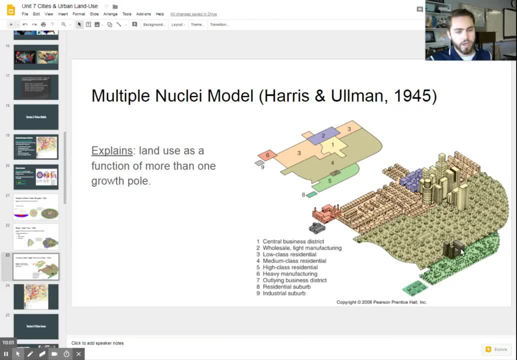 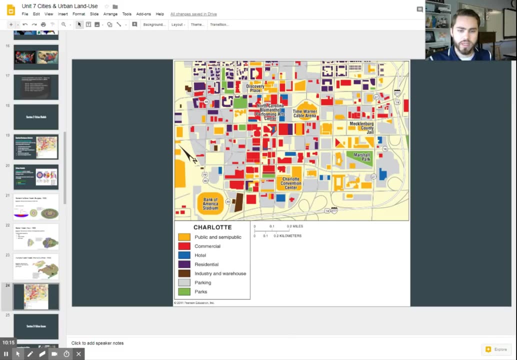 you know, or other types of services in the suburbs. this takes into account many different nuclei rather than just that single nuclei of the central business district that you see in other models. All right, so let's take a look here real quick to see if we can apply some of these concepts here. 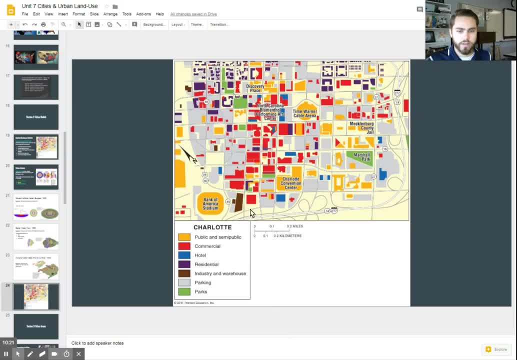 So the areas in red are your heavily commercial areas in Charlotte. So it's going to be like your central business district here in red where there's mostly high, tall skyscrapers and things of that nature. So the central business district. but notice, we have our brown, our industry here. 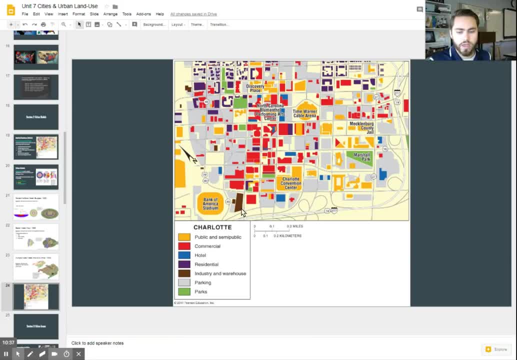 around the outside edges where it congregates, And so we can see the congregation of this multiple nuclei which is the central business district, which is the central business district, And so we have all of the sacred areas here and we can see the documentation. 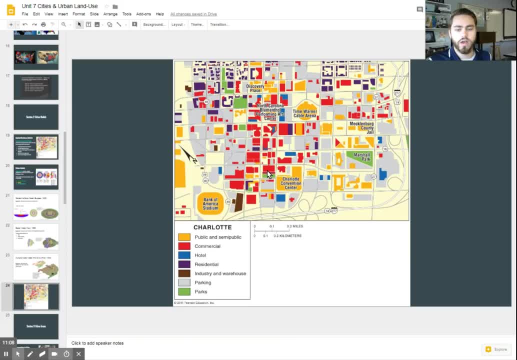 For example, I see a nuclear here. Write the same thing here. There, industry has a nuclei and these stadiums have a nuclei. these public buildings and these residences have a nuclei, and so it's not all about the central business district. there's many different areas where people congregate around and 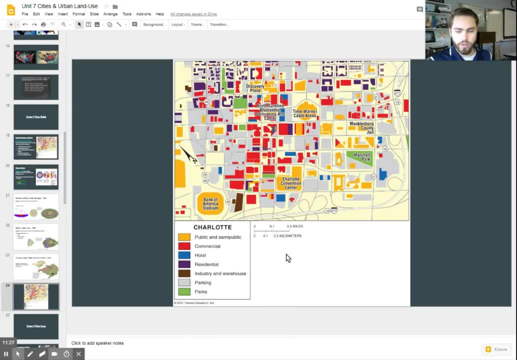 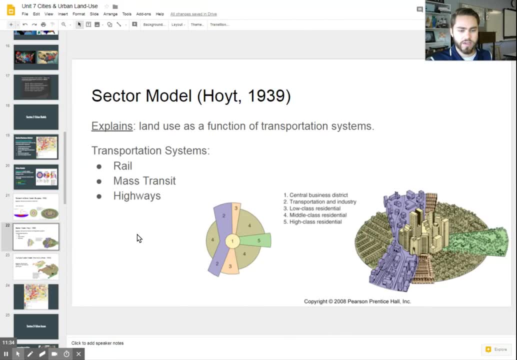 multiply multiple nuclei method or model, all right, so make sure that you understand those three models and how they help us to understand cities are set up.